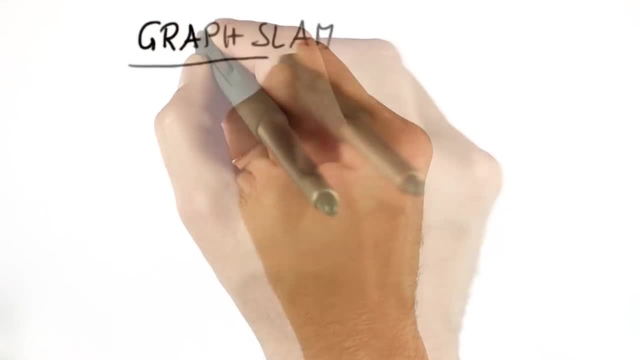 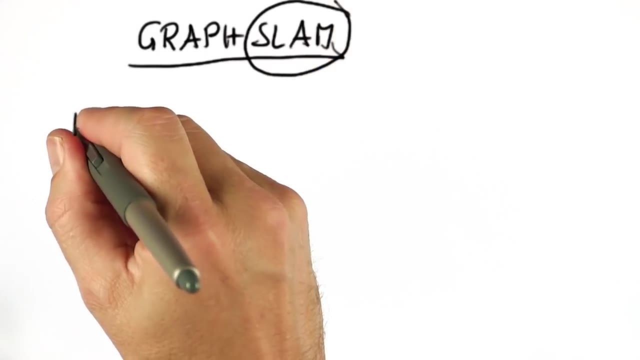 Let me take you about my favorite methods of all, called graph slam. This is one of many methods for slam and it's the one that's by far the easiest to explain. Let's assume we have a robot and let's call arbitrarily the initial location: x equals 0 and y equals 0.. 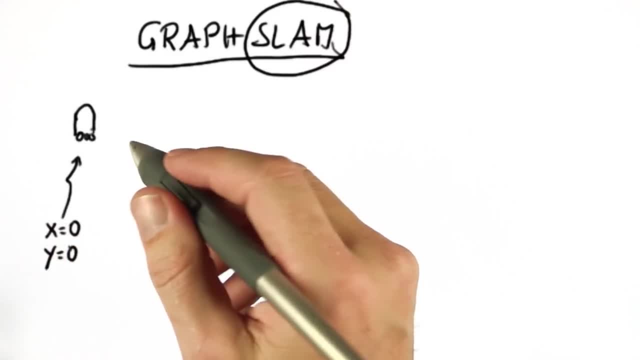 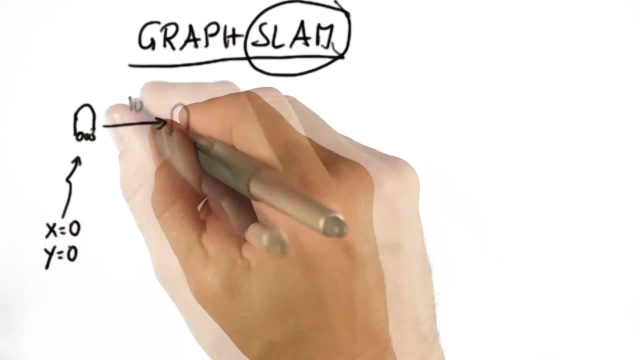 For this example, we just assume the robot has a perfect compass and we don't care about heading direction. just to keep things simple, Let's assume the robot moves to the right in x direction by 10, so it's now over here. 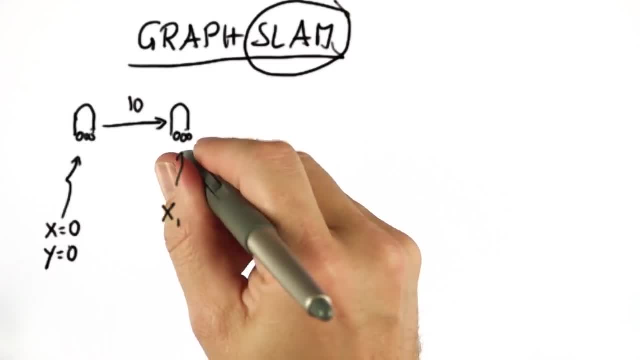 In a perfect world, you would know that x1, the location after motion- is the same as x0 plus 10, and y1 is the same as y0. But we learned from our various robotic common filter lessons and others that the location is actually uncertain. 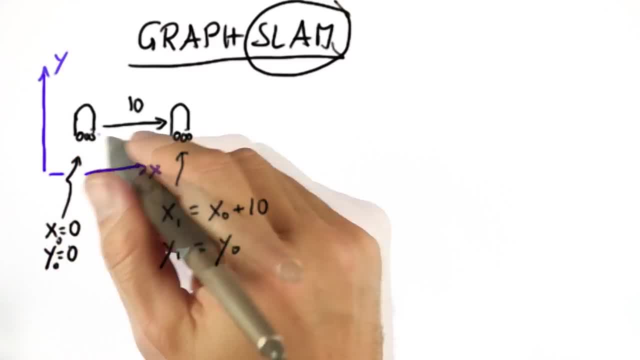 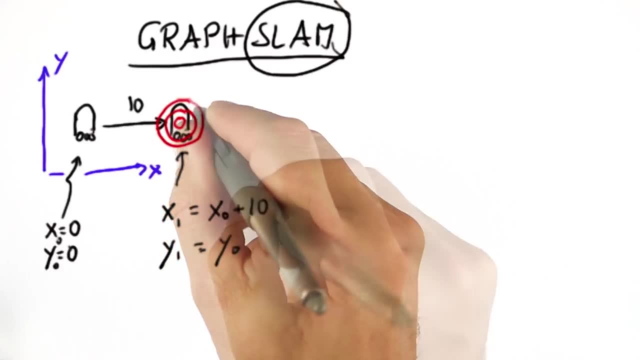 So, rather than assuming, in our x- y coordinate system the robot moved to the right by 10 exactly, we know that the actual location is a Gaussian centered around 10, 0, but it's possible the robot is same. It's somewhere else. 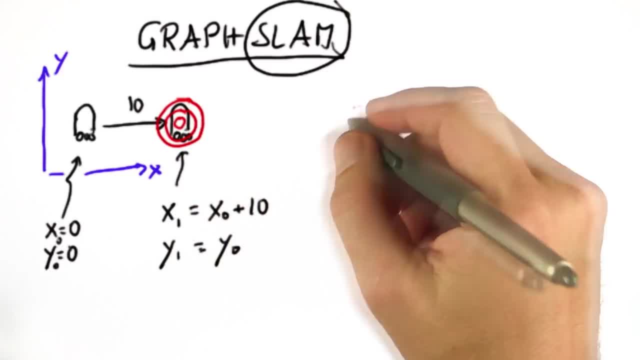 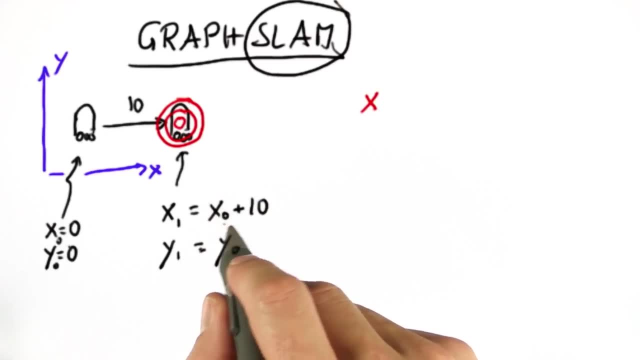 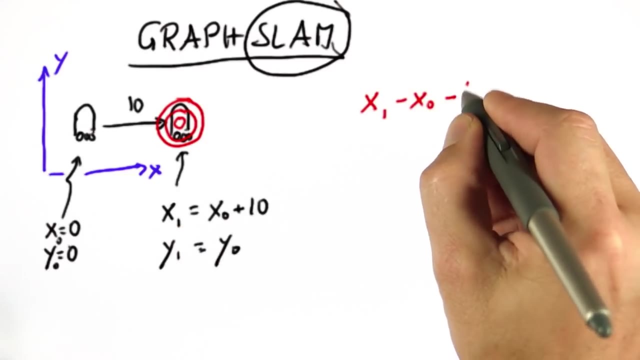 Remember we worked out the math for this Gaussian. Here's how it looks like just for the x variable. Rather than setting x1 to x0 plus 10, we try to express the Gaussian that peaks when these two things are the same. So if you subtract from x1,, x0, and 10,, 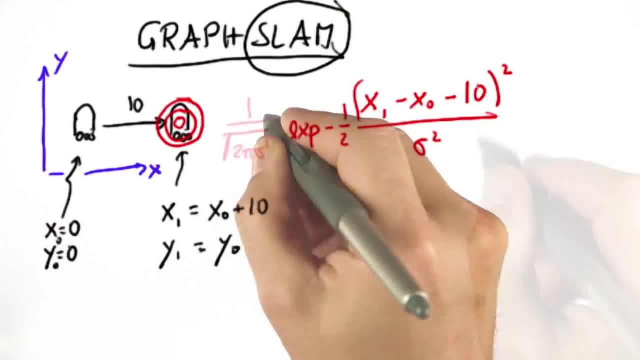 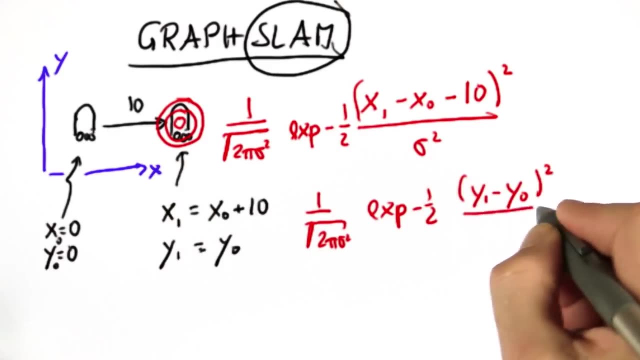 put this into a square format and turn this into a Gaussian, we get a probability distribution that relates x1 and x0.. We can do the same for y, and since there's no change in y according to our motion, all we ask is that y1 and y0 are as close together as possible. 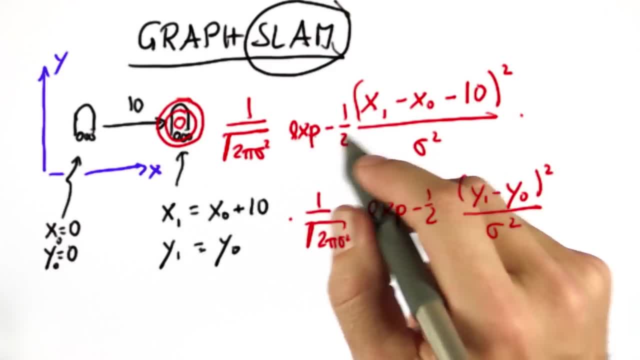 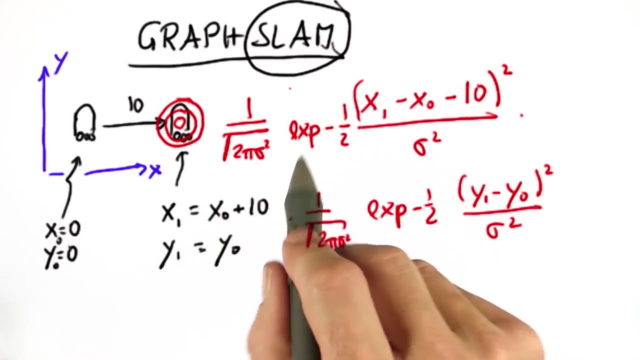 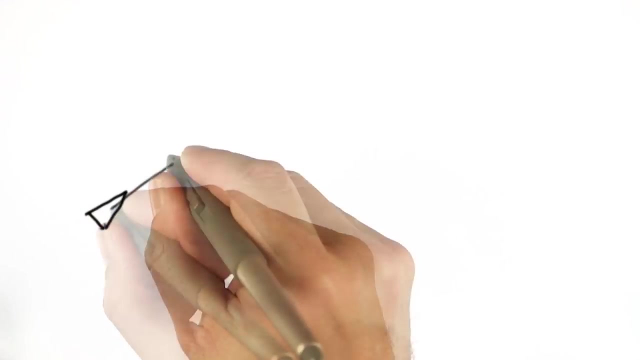 The product of these two Gaussians is now our constraint. We wish to maximize the likelihood of the position x1, given that the position x0 is. So what GraphSlam does is defining our probabilities using a sequence of such constraints. Say, we have a robot that moves in some space. 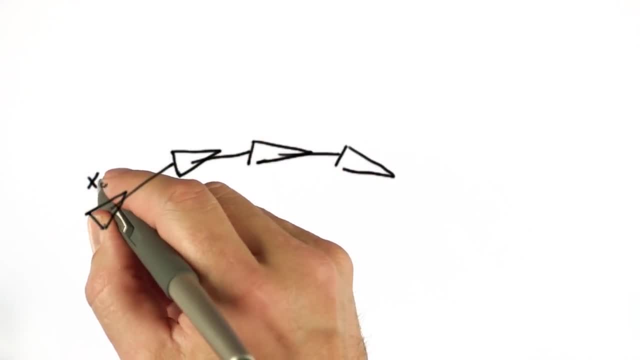 and each location is now characterized by a vector x0 and a vector x1, vector x2, vector x3. Often they're three-dimensional vectors. Then what GraphSlam collects is the initial location, which is a 0, 0, 0 usually, although here it looks a little bit different.